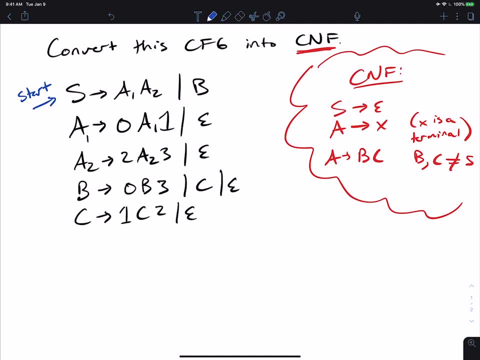 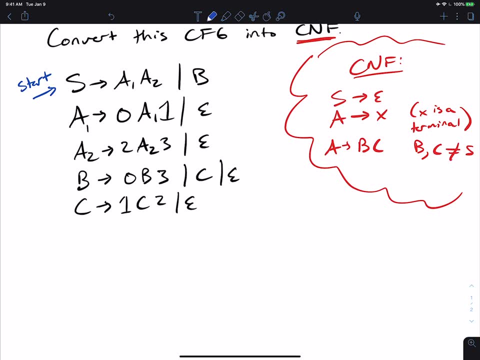 right-hand side of the grammar, So we can have: a goes to bc, so any variable can go to two variables. but we still have some work to do. So how do we actually do this? Well, we, in order to actually convert this into c and f, we actually have to do this in stages. So stage or step one is to: 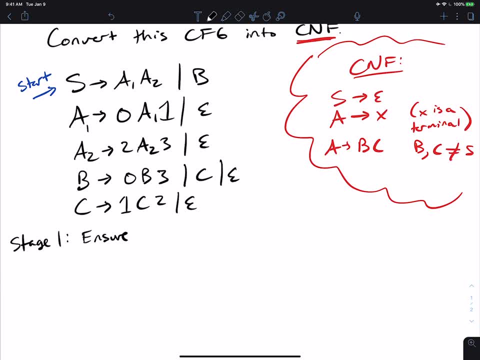 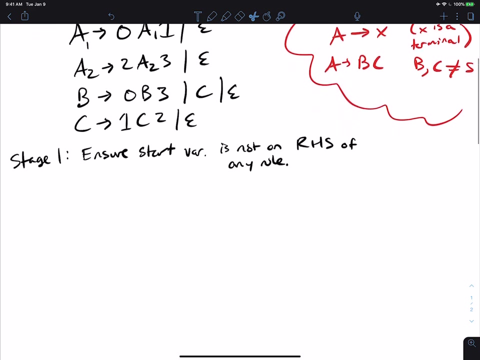 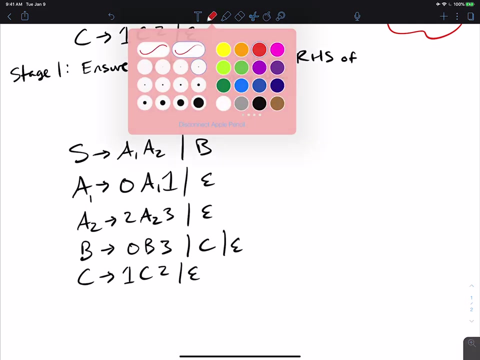 ensure the start variable, whatever it's called, is not on the right-hand side of the grammar. So what we can do to fix that or not fix it, but rather to ensure that it definitely isn't in any grammar that we consider we can add this rule: s0 goes to s, where s0 is the new start variable. 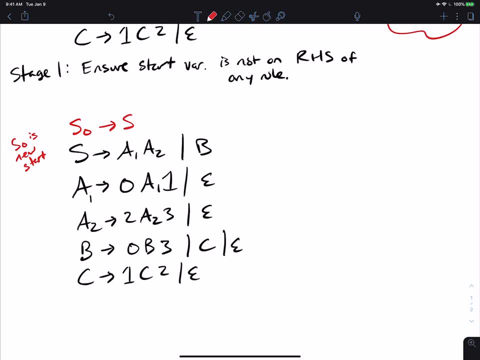 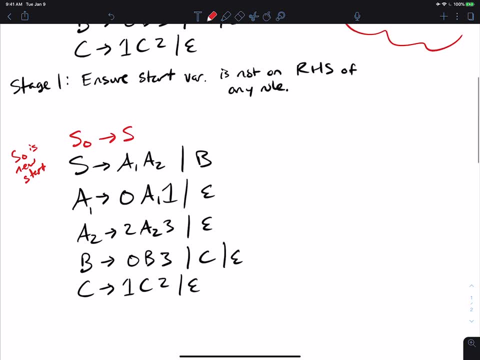 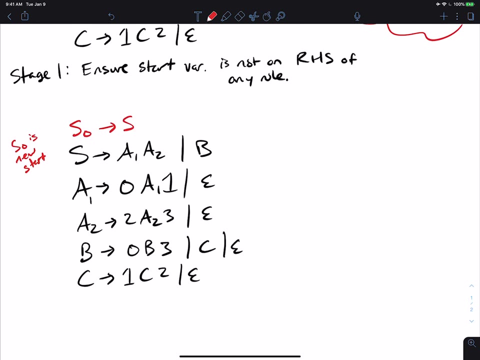 And what we want to ensure at each of these stages is that we don't change the language of the grammar. Well, we don't here, because if we had a derivation before then we can get a derivation here just by tacking on. s0 goes to s, which it has to start with anyway. And if we have a derivation, 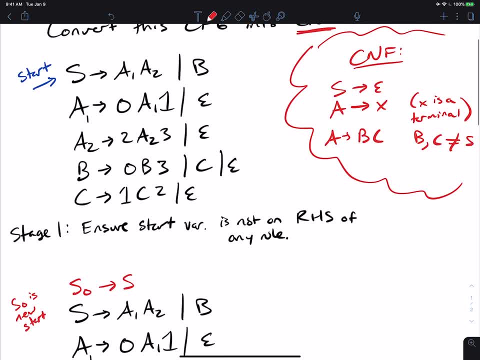 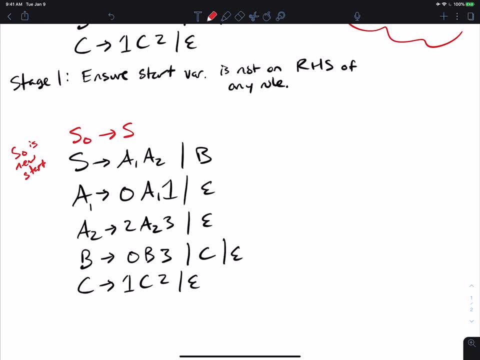 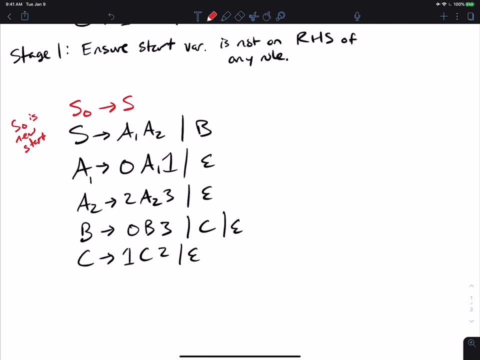 here. then we can get a derivation for the original one just by removing s0 goes to s, since every derivation in this grammar must start with s0 goes to s. Cool, So that's how we get the first stage, and the ordering of these stages matters so that we don't reintroduce problems that we have done. 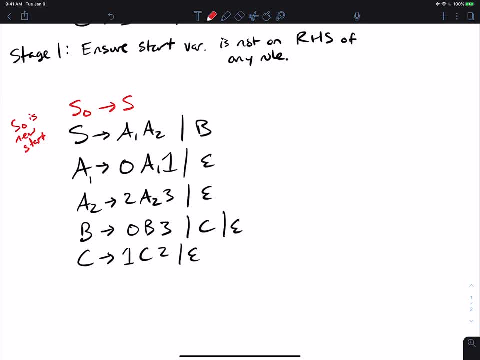 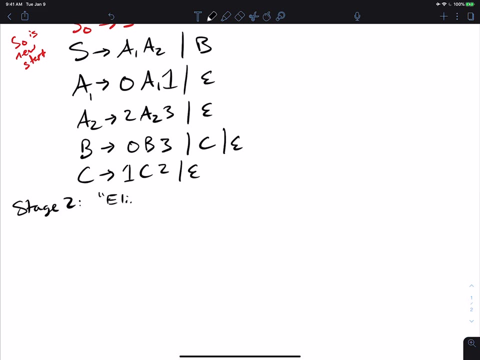 before. By doing this, we're never going to introduce s0 on the right side, so we'll never have to fix this again. Okay, the second stage- so stage 2, is to quote-unquote: eliminate all epsilon rules- possibly not for s0, the new start. 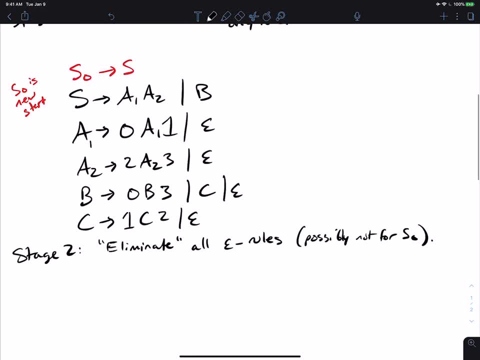 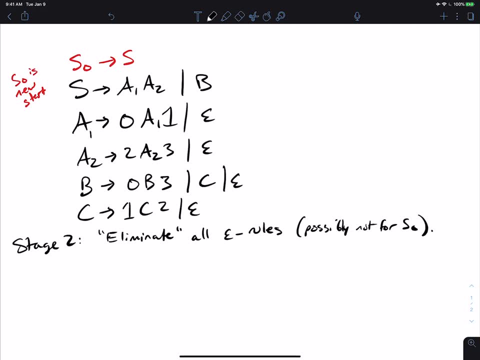 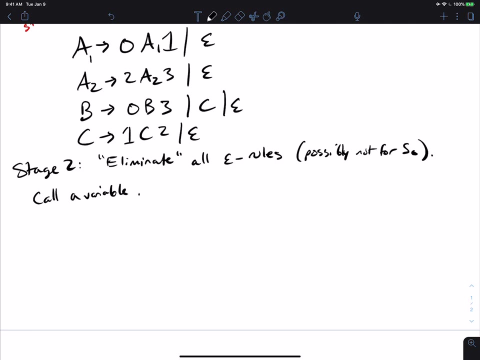 variable. So how do we actually look at this? Well, a1 goes to empty, a2 and all these other variables go to empty. So we're going to call a variable nullable if it can generate the empty string. So if it is possible to. 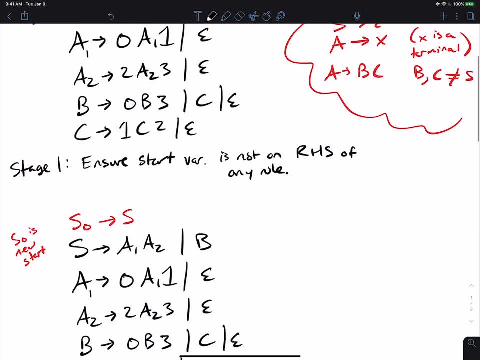 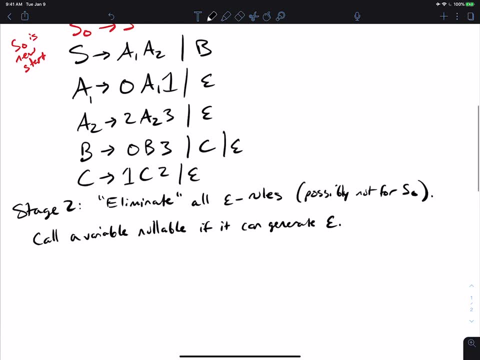 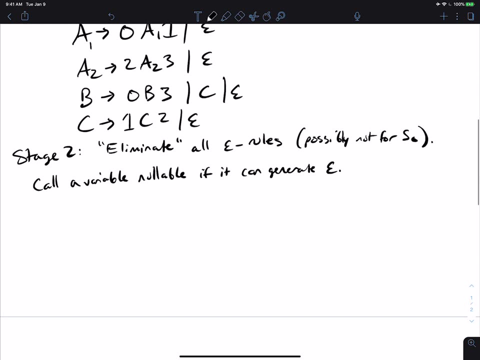 generate the empty string. well, we don't want that, because a grammar in c and f should only have the start variable making empty. So well, we know that a1 can is nullable because it can make the empty string directly. So I'm going to make a list of nullable variables. 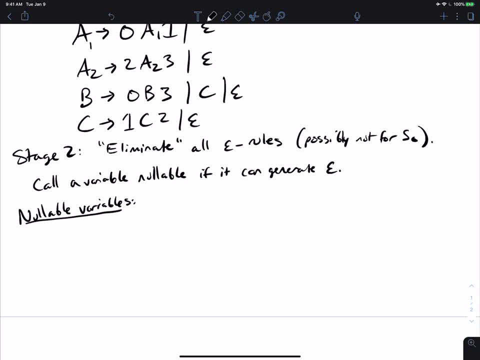 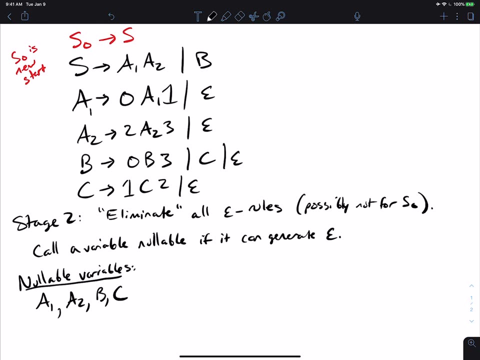 right here. Well, a1 is clearly on that list, a2 is also on that list, b is on that list and c is on that list because all four of them make empty. But take a look at s. Well, s can't make epsilon. 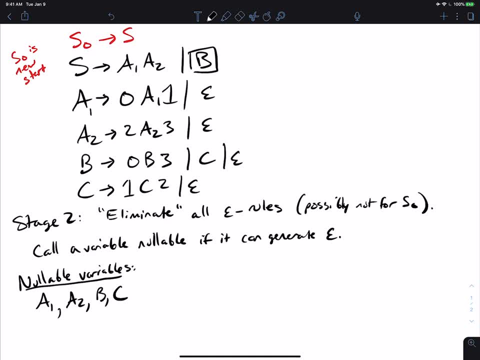 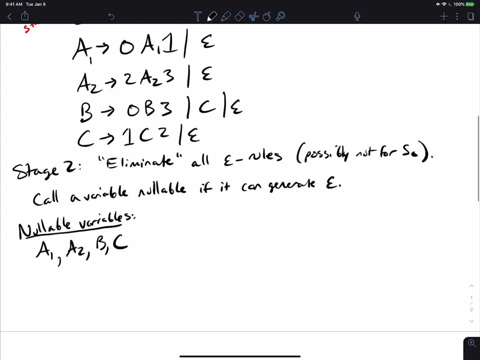 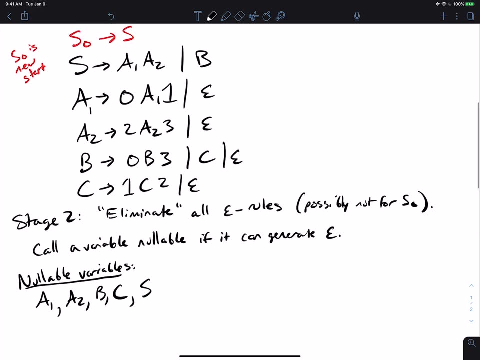 directly. So a2 right here can make epsilon directly, And because of that we know that s can make epsilon directly. So s is a nullable variable, I mean indirectly. s is a nullable variable because it can generate epsilon eventually, And s0,, for that same reason, is also a nullable. 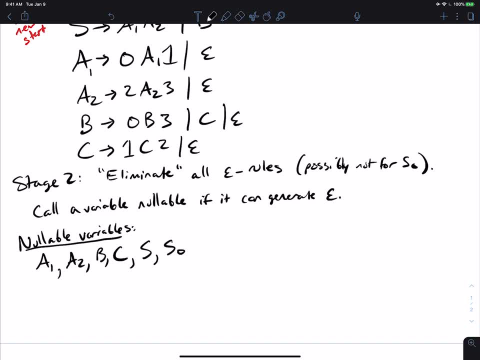 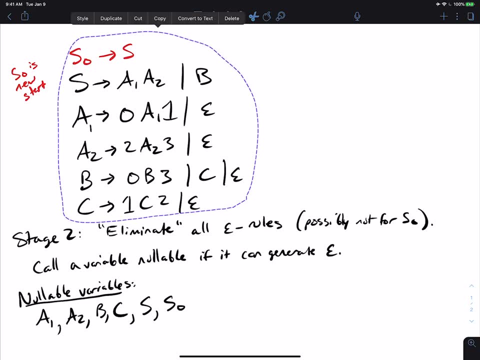 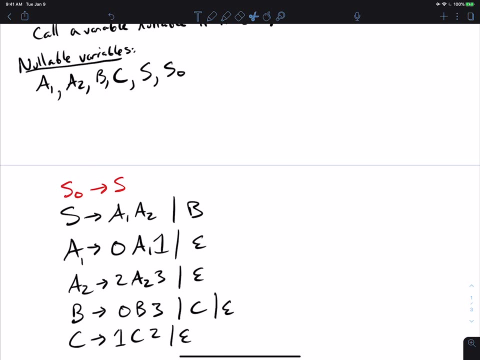 variable, So every variable is nullable in this grammar. So how are we going to, you know, remove these epsilon rules in this grammar? So what I'm going to do is I'm going to copy these down down here. Well, we know that s0 is nullable, meaning it can make the empty string. 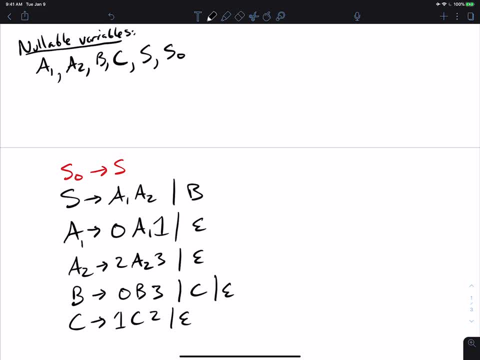 So in the final grammar, we want it to make the empty string, because we know it can So here and because we need to have the start variable, making the empty string directly and no other way. we got to have or epsilon upstairs, Well. so then, how do we handle these down here? Well, 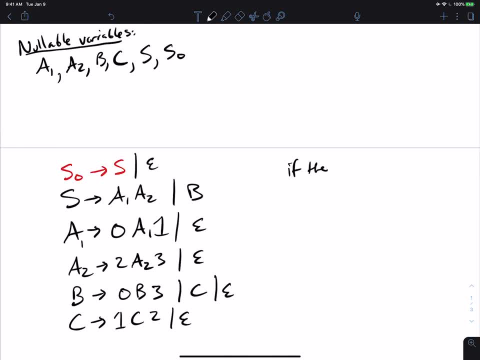 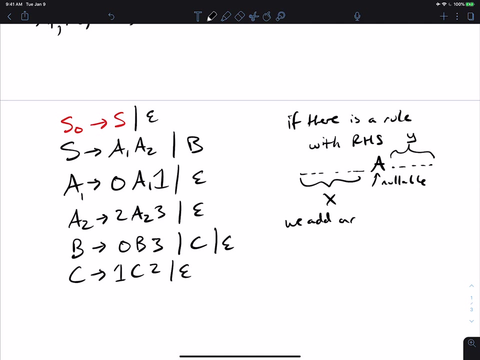 what we're going to do is if there is a rule with right-hand side something in an a where this is nullable, So maybe let's just call this part x, whatever it is, and then maybe this part y, Then we add a rule. 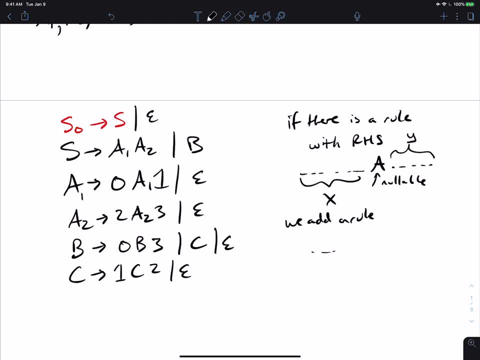 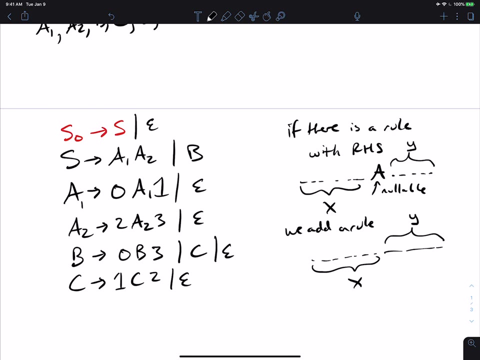 which is the x part here and then the y part here, where there's no a in the middle. So we're, basically, we're adding a rule to simulate as if a went to empty Or it eventually generated empty, without actually generating it directly or indirectly. So we're. 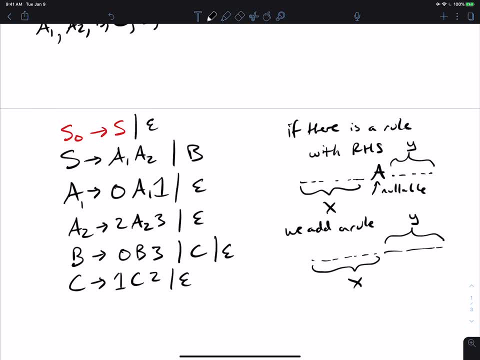 adding an additional rule to handle the case of whether a makes the empty string. It might not, but in the case that it does, we have another rule to help us with this. So let's see how are we going to do this. So, the way that I like doing this, you can do this in any order you want. 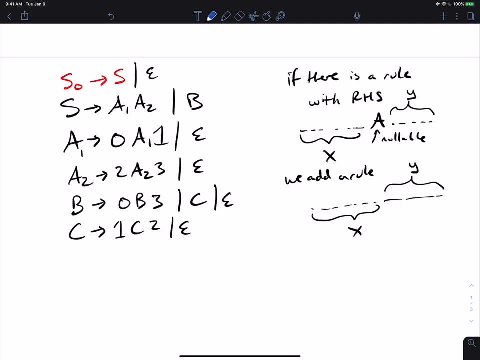 but let's just start at the bottom with the c rules. Eventually, we're going to get rid of these epsilon rules other than the one with s0, of course. So what we're going to do is: well, let's look at this rule right here. Is there a nullable variable? 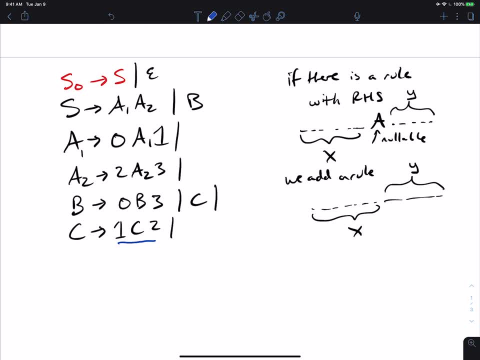 in there There is because it's c. So we're going to add a rule where c is taken out. So we have 1 and 2 here because 1 and 2 are terminals, and then we don't have to do anything with those. 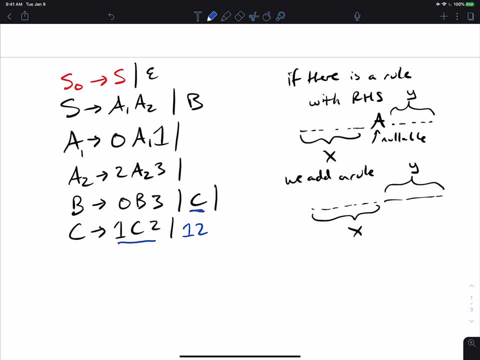 B is nullable. Well, this rule: if we remove c because c is nullable, we would add epsilon here. but we don't want to have that because we don't want to introduce epsilon rules. So we're going to ignore this one And then for: 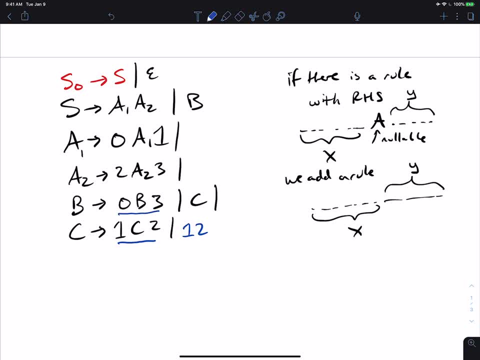 this rule. right here, we're going to have exactly the same idea, which is 0, 3.. Then, for the a2 rule, we're going to have a2 variable, excuse me. Then we're going to add 2, 3.. a1,: we're going to add 0, 1.. 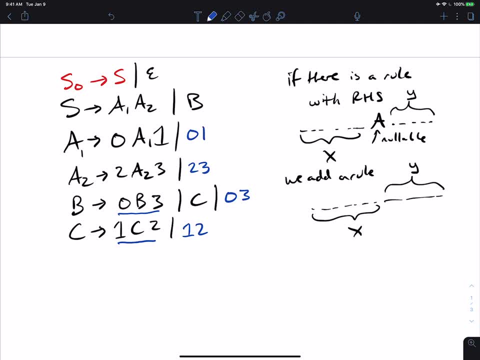 And then- so this is for this rule- it gets interesting. Well, this one for b is the same scenario as before, so we're going to ignore it For this one. well, it could be that a1 goes to empty and a2 doesn't, So we're going to add a rule for the case of where a2 goes to empty. 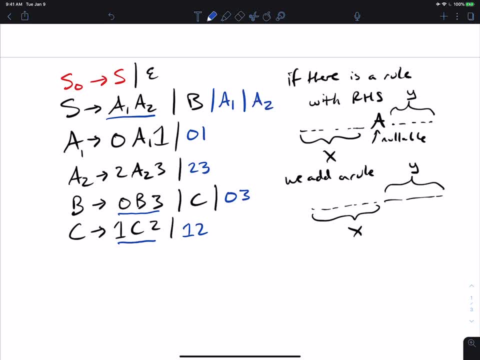 as well as the case of where a1 goes to empty. So any choice of a variable dropping out, so to speak, from the right-hand side of the rule. we're going to add all of those possibilities, every single one of them. Okay, so I think we have removed all of the epsilon rules. 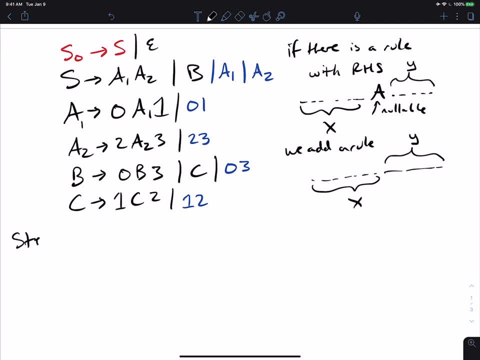 now. So we're ready to move on to step or. my notation is stage. stage three, which is to quote-unquote eliminate unit rules. And, by the way, the reason I say eliminate in quotes here is so that I don't. 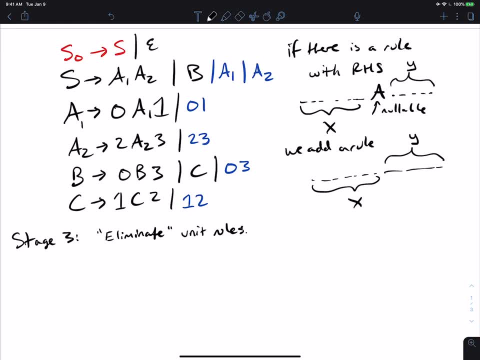 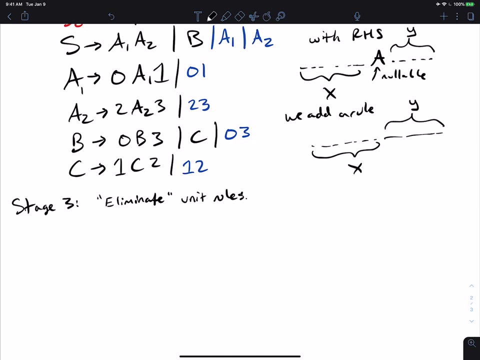 want you to literally eliminate the rules, the epsilon rules, because that will actually change the language. What we're doing is we're simulating those rules with other rules and then eliminating them later, So we're not changing the language at any point. Okay, so what is a unit rule? Well, 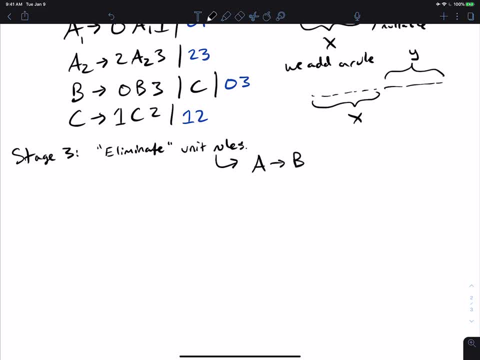 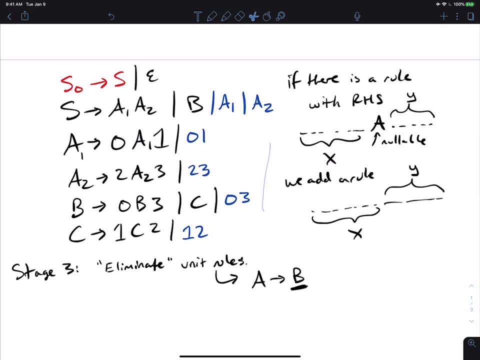 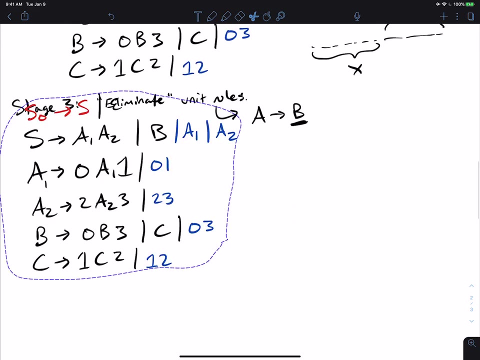 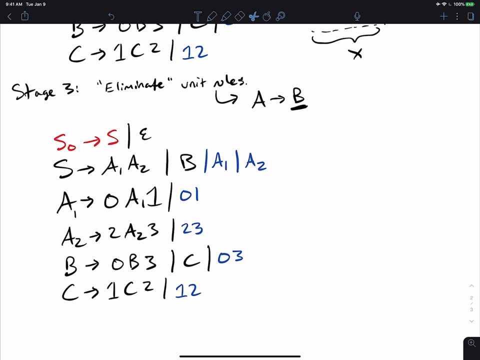 unit rule is something of the form a goes to b, so where there's exactly one variable on the right-hand side. So let's copy our grammar down and then try to eliminate unit rules. Again, I don't literally mean eliminate the rules, I mean just try to deal with them so that you're simulating them with other. 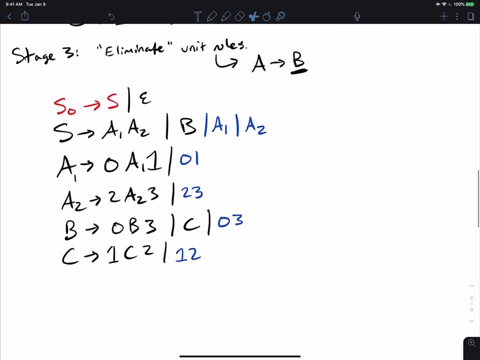 rules. So the way that I like doing this is: well, notice that the variable c down here has no unit rules, because everything on the right-hand side has terminals in it. So let's see, let's go up a level. Well, we see that there's a rule- b goes to c right here, which is a unit rule. Well, c has no unit. 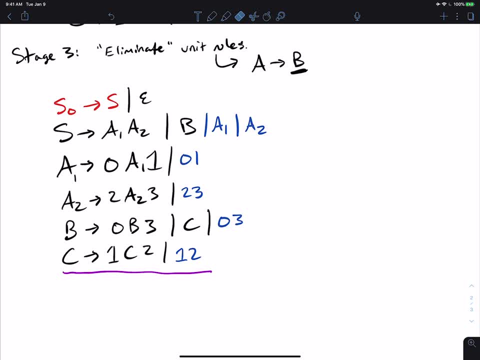 rules attached to it. So the way that I like doing this is to eliminate the unit rule, literally eliminate it, move this over, and then what we do is we copy all of the rules associated with c back up to b, So like this: 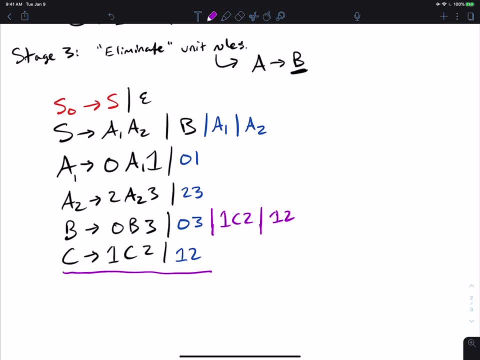 Okay. so the reason for doing this is we're simulating the unit rule with directly doing one of the rules of c without having a unit rule attached to it. So we're simulating the unit rule with directly, without having a unit rule attached to it. So the way that I like doing is we're 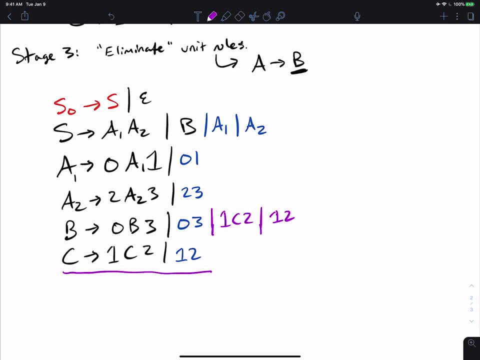 simulating the unit rule with directly doing one of the rules of c without having a unit rule attached to it. So basically we're short cutting our way to the right-hand sides of c because there was a unit rule there. So we're done with b now. a was no unit rules. a has no unit rules. s had a. 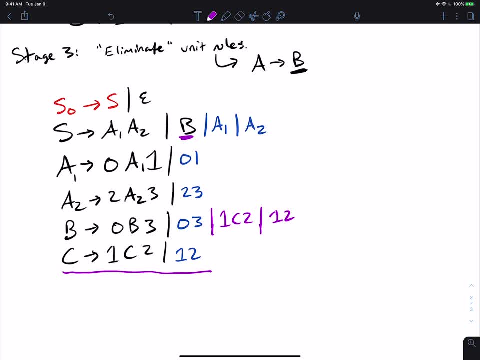 unit rule, which was b. Well, thankfully, we've already done the work for b, So b has no unit rules. So let's copy all of this with a unit rule, MATH 원. Let's copy all of this with a unit rule: MATH Macht. 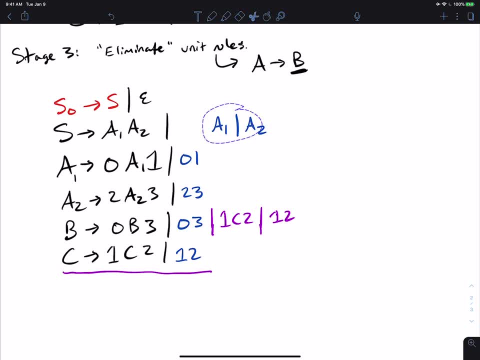 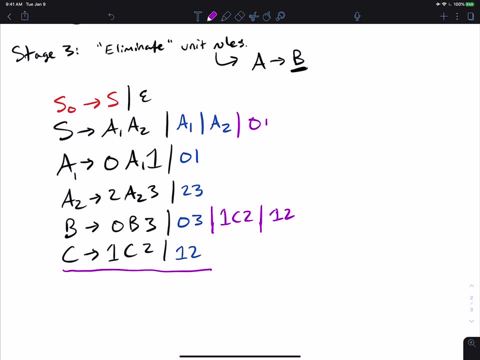 53.. those rules up by moving these over and then copy the right-hand side of b over, which is 0, b3, or 0, 3, or 1, c2, or 1, 2.. And there's another unit rule with s0,. 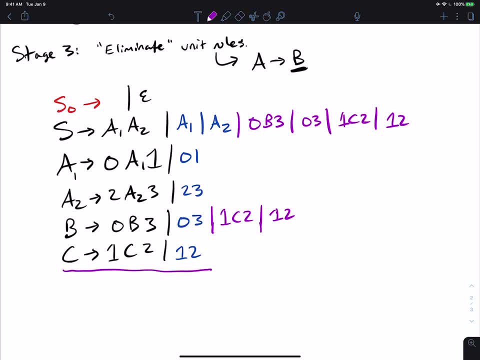 and what I'm gonna do here to make this easier, so I don't have to copy and paste everything over and over and over, is to say, all of this stuff with s also goes here. So s0 is gonna have exactly the same rules as s, except it has an or. 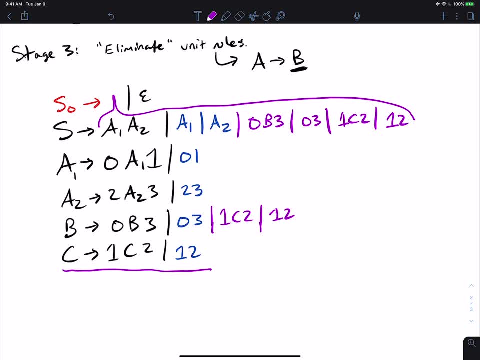 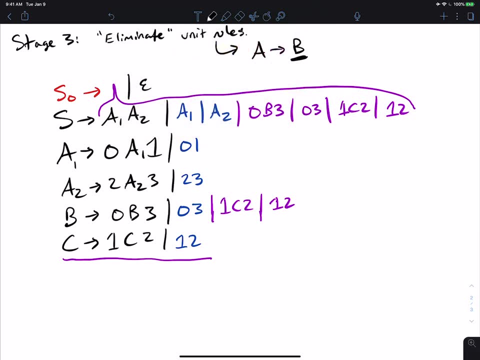 epsilon up there. Cool, So great. we're almost there, but we have two more stages to go So we notice that we're kind of on the way there. Oh, oops, I forgot. I forgot to copy the rules for a1 and a2 up, My mistake, So I need to fix that. So 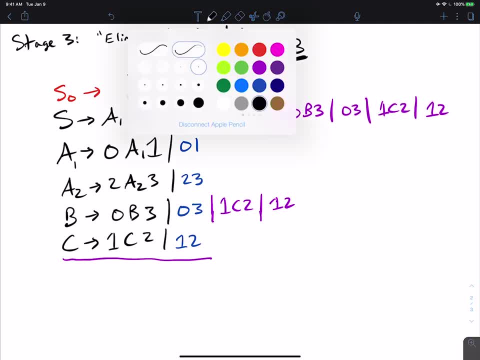 I need to make room for those. So let's see: So we have a1, has 0, a1, 1, or 0, 1, and then a2, because we had a unit rule there- 2,, a2,, 3, or 2, 3.. 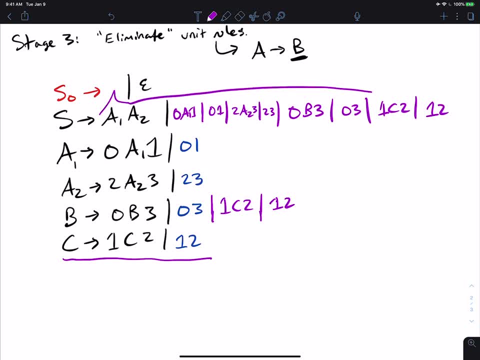 So it was quite a long right hand side. good thing i caught that. So yeah, so we're almost there. well, we have some cases of where we have two variables on the right-hand side and nothing else, which is great, but we. 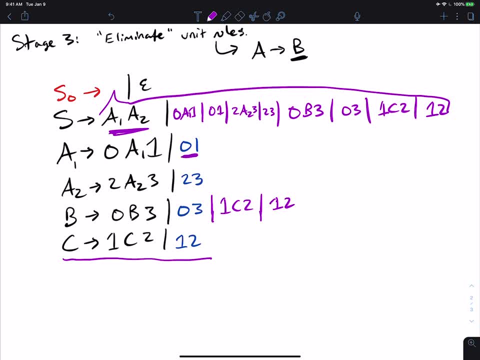 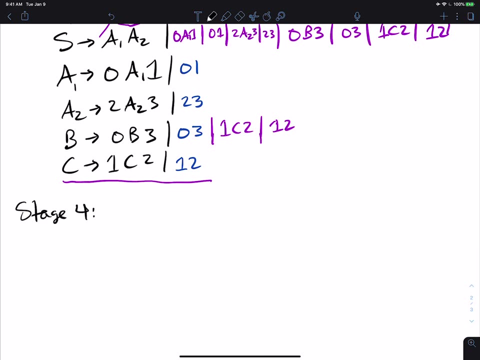 sometimes have multiple terminals or we have a mix of terminals and variables, which is something that we don't actually want, obviously, because it's not a grammar in CNF. So the fourth stage, stage 4, is to ensure I can spell, ensure the right-hand side is all. 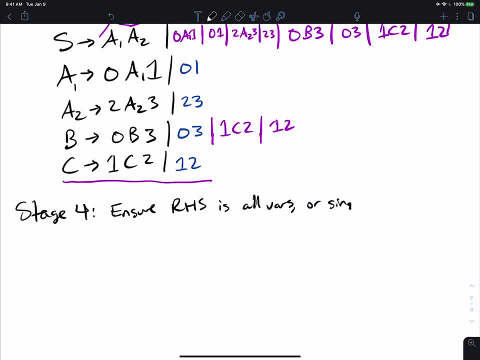 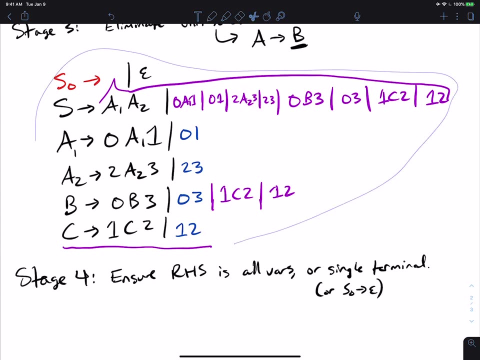 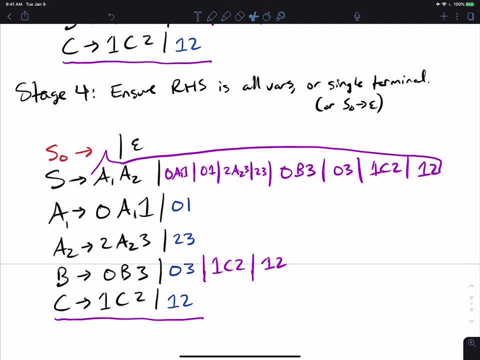 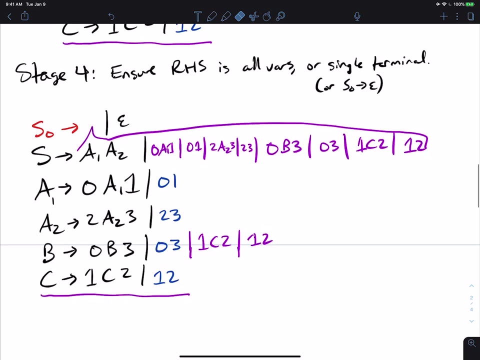 variables or single terminal or s 0 goes to epsilon, which we're not going to modify. so what are we gonna do here? I'm just gonna copy everything down so that we can work with it. okay, so what we're gonna do? oops, I didn't mean to delete. 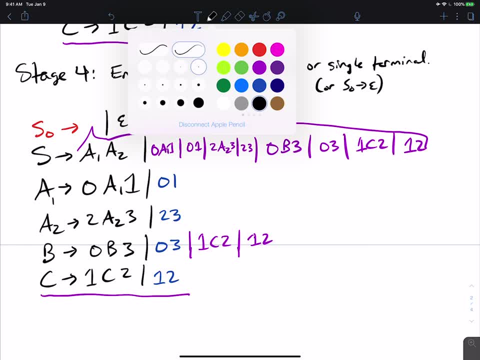 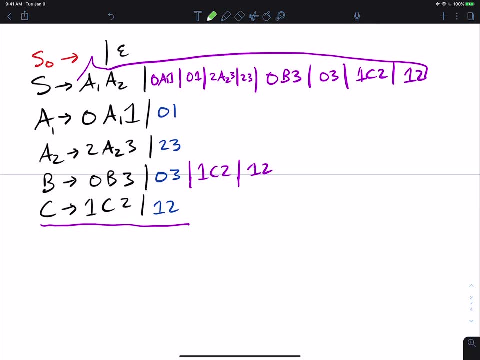 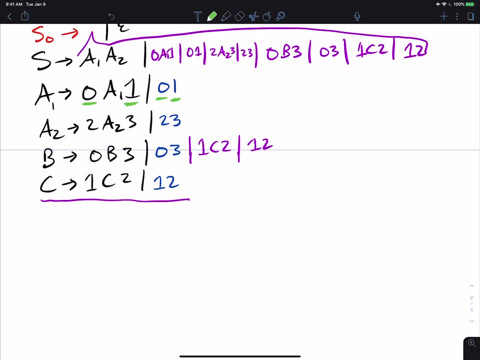 that. so let's say we're gonna go to a I don't know green color and what we're gonna do is we're going to fix these occurrences of terminals and turn them into variables. so I'm gonna make a variable called u 0, which only makes the terminal 0, which is 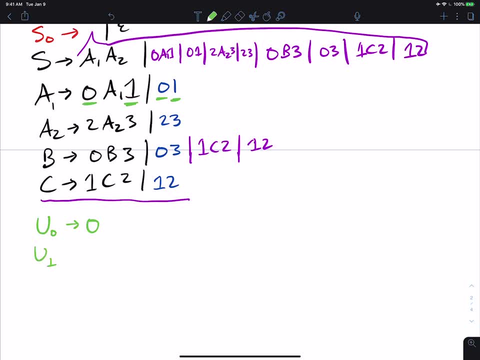 fine, because it's a grammar in cnf and we can have exactly one terminal on the right-hand side, so, and I'm gonna have another one for one, and what I'm gonna do is simply just replace every occurrence with a new one, and I'm gonna go ahead and do that, and I'm gonna go ahead and. 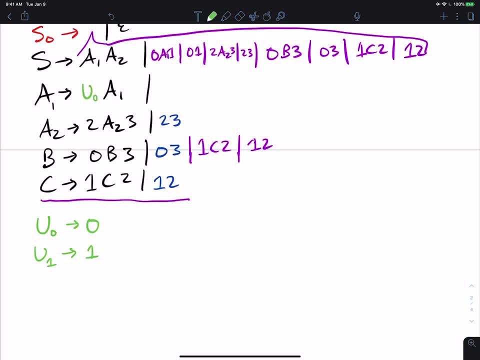 you will notice, I don't have any new terminals until I validate all of my terminals, but all I have is a girlfriend that's here. so if I never have any terminals, in this case I could just reallocate them into subur bands. huh, I think that doesn't have to do that. so if I have to fix the terminals, I just 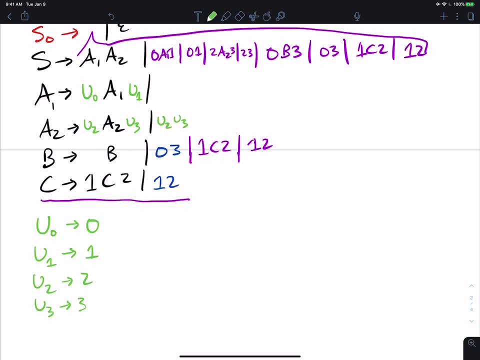 need to use an Take Action in here, and then it's going to ask's me to reallocate what do I need. so I'm gonna go ahead and do an take town and I want to tara see a U3, and then 1, 2, 1, 2, U1, U2, U1, U2.. This one, this one, U1, U2, U1,, not across- U1, U2,. 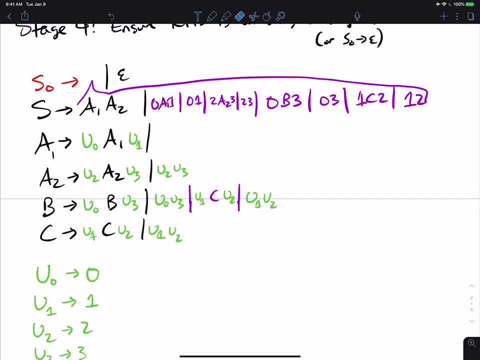 and then now the big boy which is U0, U1,, U0, U1,, then 2, 3, then 0, 3.. And then finally, 1, 2.. This is definitely the most labor-intensive one step of them all. 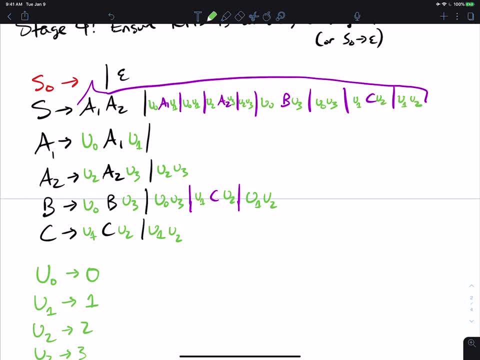 Okay, I think I got those all good and I don't see any other versions. And, by the way, if you have a right-hand side with exactly one terminal, you don't change it into a variable, because then you would be introducing a unit rule, which is something that we 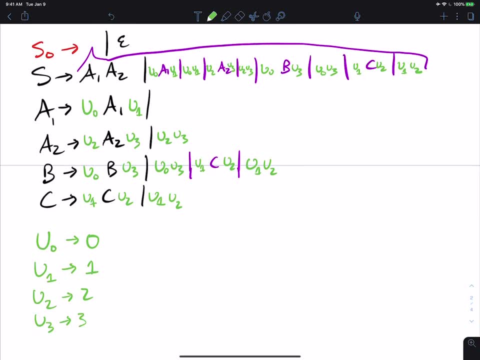 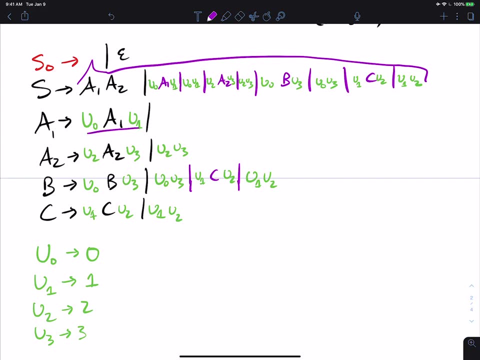 obviously don't want anymore. Okay, so we're almost there We have. most of the right-hand sides are okay, except now we have three variables on the right-hand side and we want to get it down to two. So the fifth and final stage. so stage five. 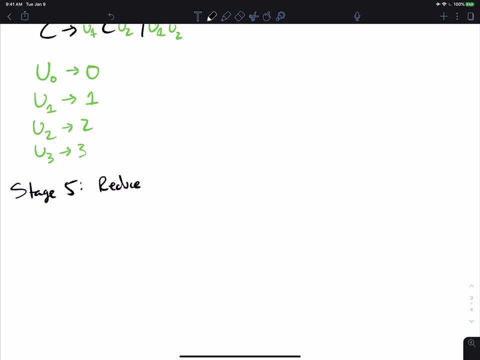 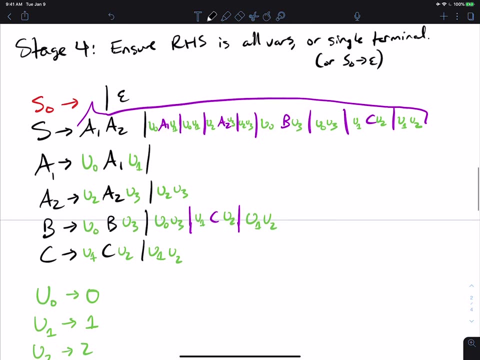 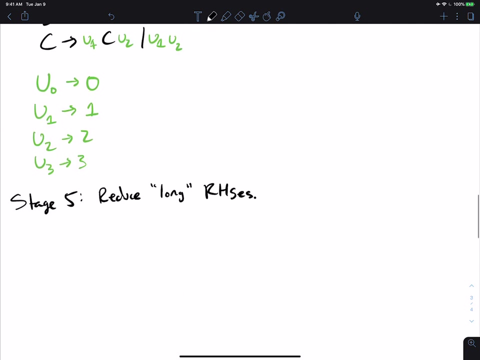 is to reduce the quote-unquote long right-hand sides. So from stage four we guarantee every right-hand side is all variables or a single terminal. So by long here I mean at least three variables, because if it's two variables then there's no need to change it, And if it's one variable, well, 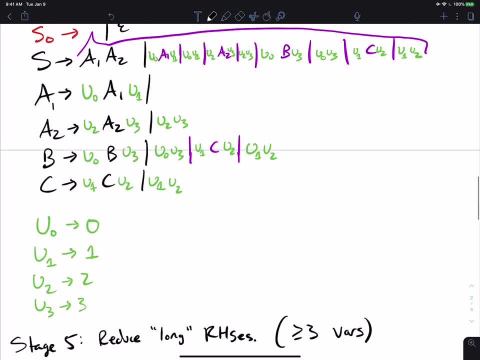 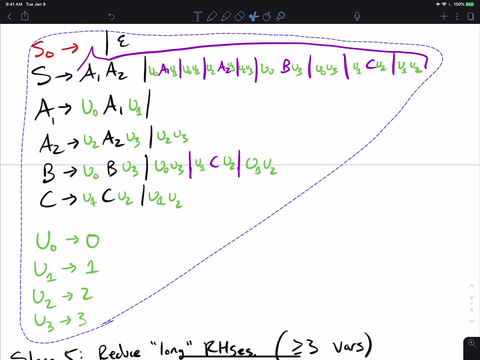 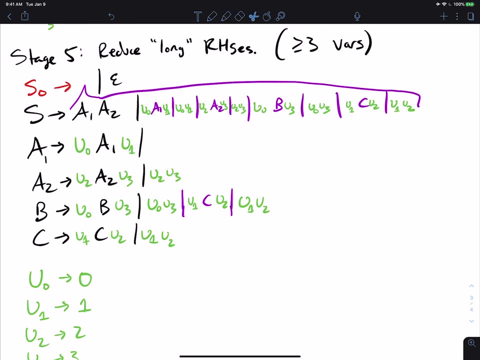 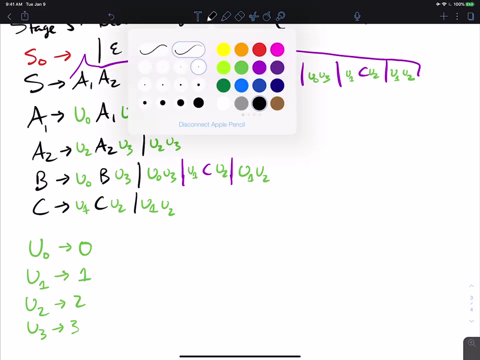 that's not possible because we've eliminated those already. So let's copy this big grammar down So that we can finally get this big boy into CNF. Okay, so what we want to do is again, let's simulate a rule with other rules. 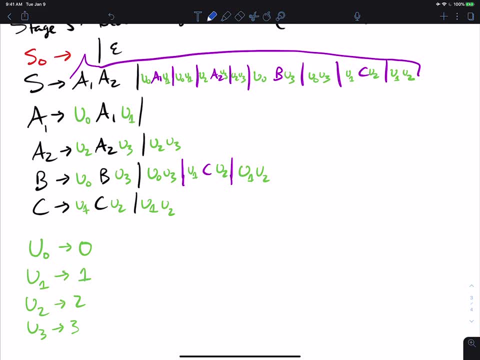 So what I'm going to do here is I'm going to substitute U0A1.. You don't have to do it in this particular way, but this is just one way to do it. So let's say I'm going to replace these two variables with a different variable. I'm going to 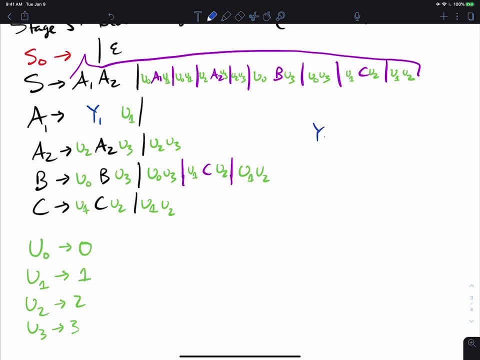 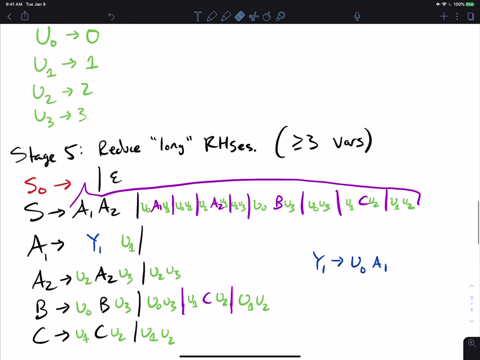 call y1 and y1 is going to make u0, a1. and notice what we did here. we reduced three variables into two and we guarantee to produce the same rule because if I take a1 then I'm going to. oh, did I have a mistake? I might have had. 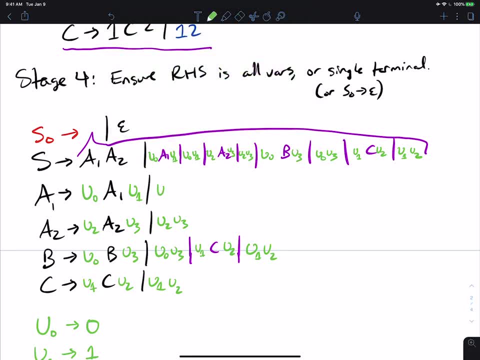 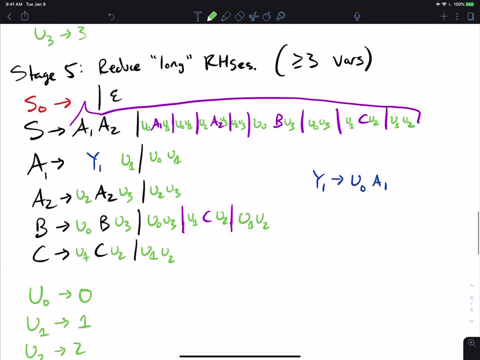 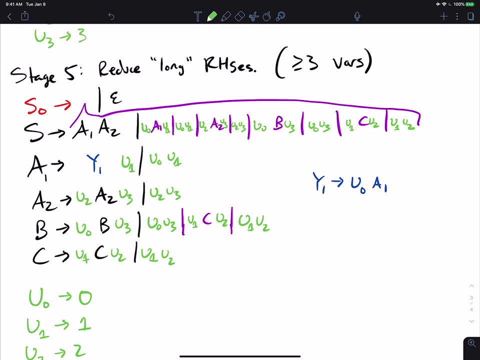 a mistake. so this should have been u0- u1 and this one should have been u0- yep. sometimes we make mistakes too. okay, so I would, if I chose that rule before, well, I would have had u0 a1- u1. well, if I chose it now. 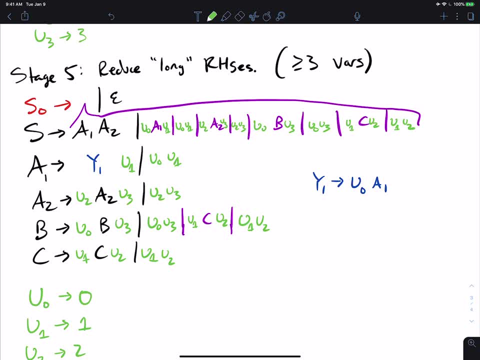 well, right, at this point we are babe happy because we can guess that we still had b1, b2, right? so if I chose that roll before, well, I would have had u0 and alcoholic. I would have to do y1, which the only thing it can make is u0, a1. So therefore, we are simulating. 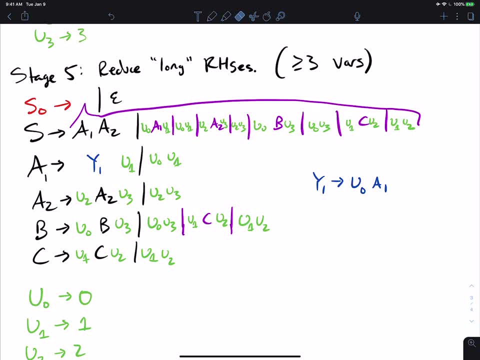 the original rule with another rule, And I can replace every other version of it again with y1.. Make the ones look nice And let's see: are there any other ones? I don't see any, So let's make a y2 to make u2, a2.. And replace them in their appropriate places.